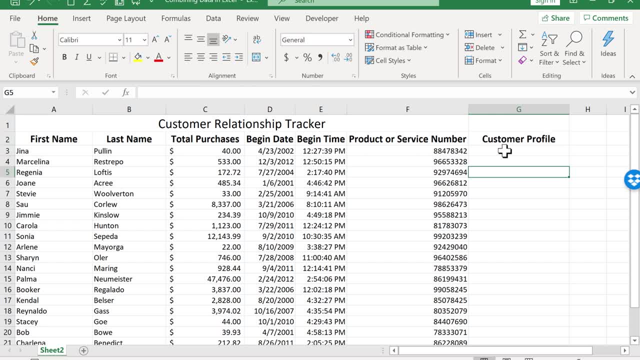 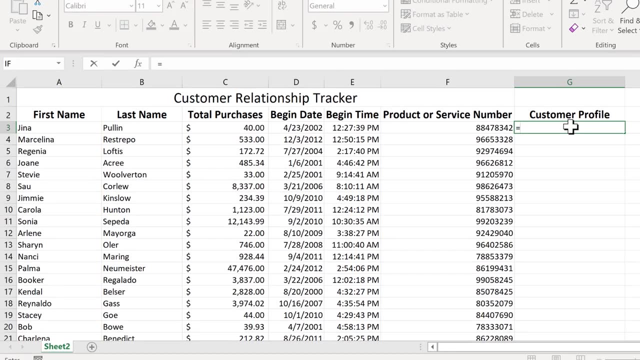 And it makes the format the same. Okay, so watch how I can do this, how I can add the word Gina to the word Pullen and let's say the total amount of purchases that they've made in dollars. So I'll just click here in cell G3, and I'll type equals. So this cell equals and I want it to equal Gina. 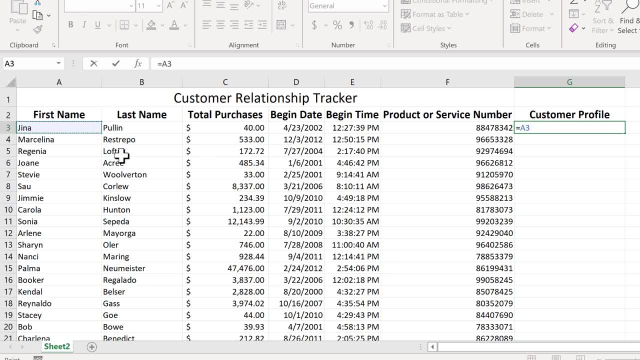 So I click on Gina and then I also want it to include the word Pullen. But if I click on Pullen it changes. It changes to B3. So what if I click Gina plus Pullen and hit return? Look, Excel doesn't. 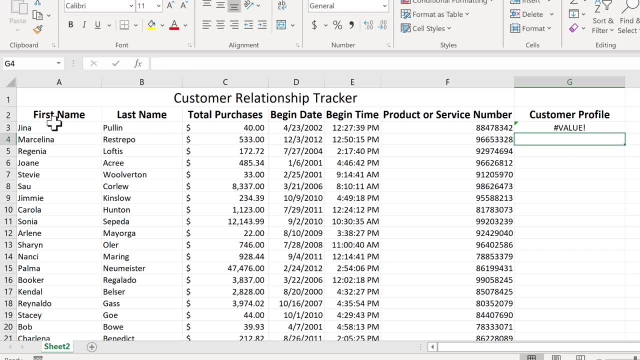 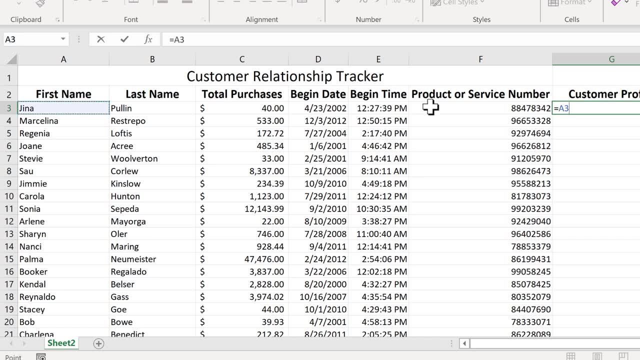 understand It doesn't seem to compute. You know how do you add a name plus another name. So the way you do this properly is you type equals, click on Gina, and then you type an ampersand, or some people just call it the end sign. So A3, ampersand Pullen. Now watch what happens If I tap enter or 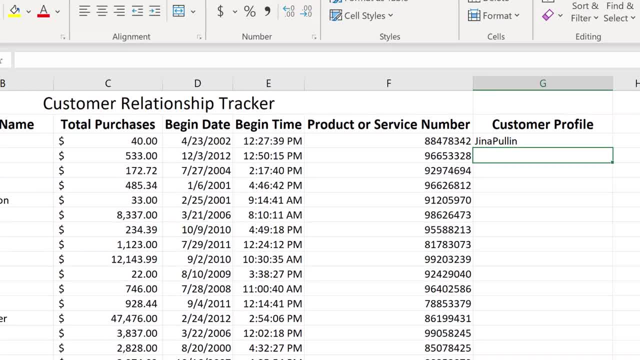 return on the keyboard, I'm going to be able to add a name. So I'm going to be able to add a name. It says Gina Pullen. It combined the contents of cell A3 with the contents of cell B3.. Now there's. 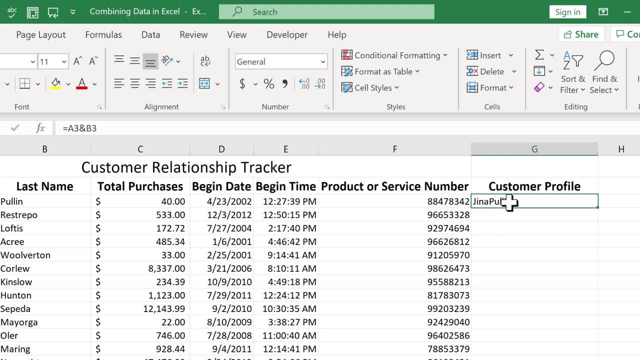 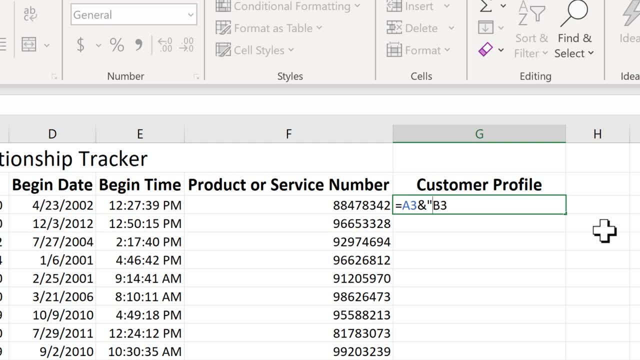 a problem here. There's no space between Gina and Pullen, So let's fix that. All I have to do to put a space in is after the ampersand type in quotation marks a space using the space bar. 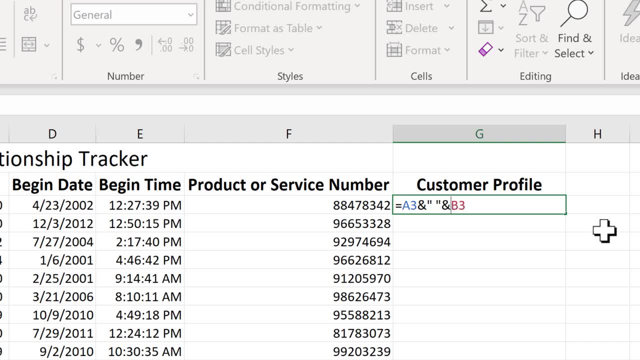 and then quotation marks again and then type an ampersand again. So what this should do is it forgets all the singled out alcanzations. what was missing is something that it ended up with a space, and then it connects that with whatever's in B3. So I tap return or enter on the keyboard. 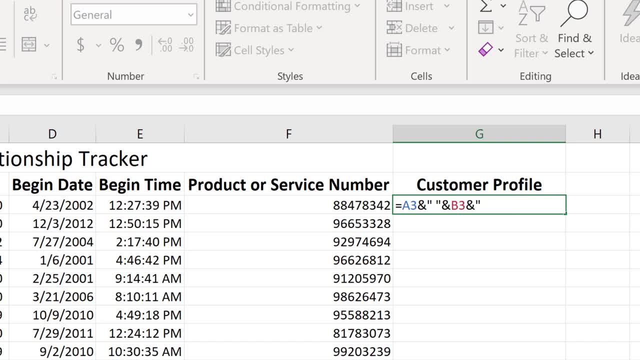 and it worked. Now let's change it even more. I want to add now the total purchases, So I'll just add another ampersand and I should probably put a space in there again or maybe a colon. Let's try a colon- And then I put the close. quote another ampersand and maybe I want another space in there. So I put in: quote space closed. quote another ampersand from B3 to B: Etch: Talk about live chat R. 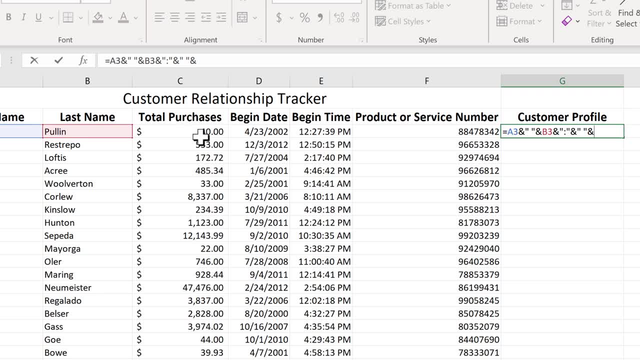 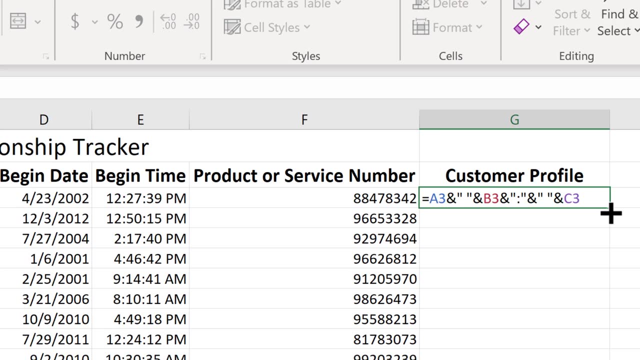 ampersand, and now i'm going to click on the total amount of purchases here and tap enter on the keyboard or return, if you're using a mac, and look what we have. gina pullen 40. if i really wanted to get picky with this, i could go in and add a dollar sign. so after the last ampersand, quotation marks. 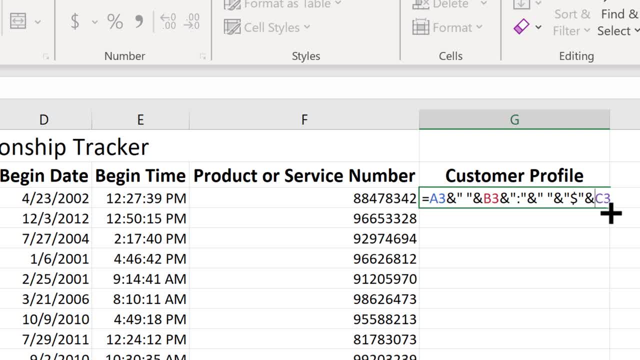 dollar sign quotation marks. i'll need another ampersand tap, return or enter on the keyboard, and now that looks just how i want it to look. so this is a very simple customer profile, but it lets me know the names of the customers who have purchased the most from us over the years. 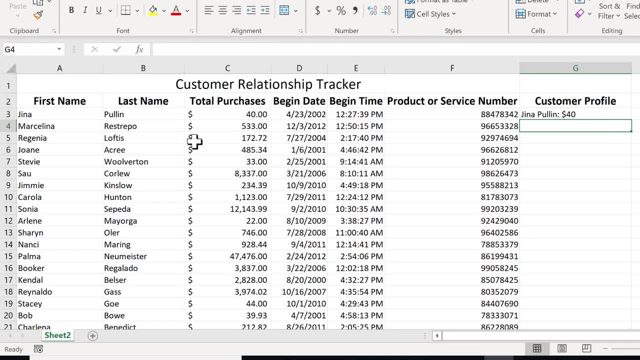 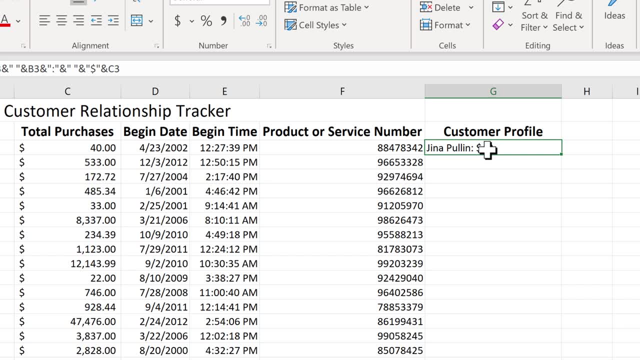 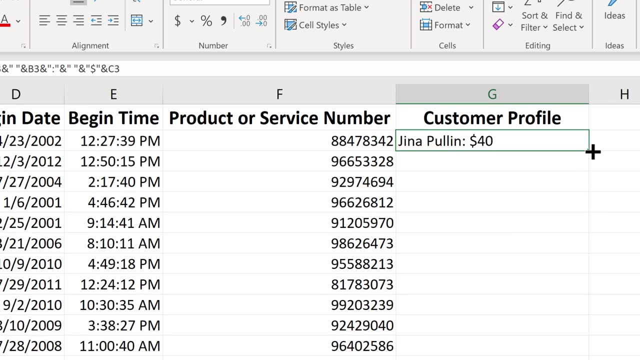 now, unfortunately, i'm gonna have to do that again for every single one of these customers, right? well, actually, no, all i have to do is click on gina, pullen forty dollars and go to the autofill handle. i'm going to zoom in on this a little bit, but you can see it here anytime you've clicked on. 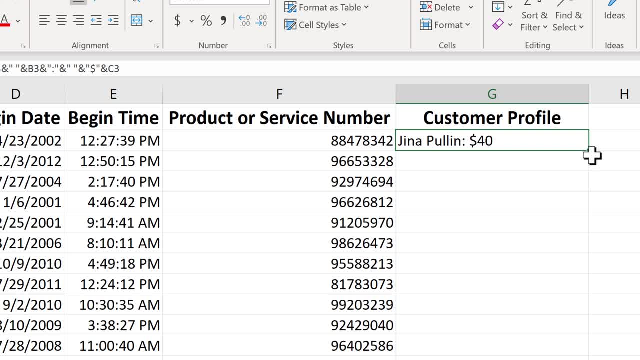 a sign. you'll be able to see the number of customers that have purchased the most from us. in the lower right corner of that cell there should be a very small square. you can see it there. it's green, and that is the autofill handle, and what it does is that it copies. 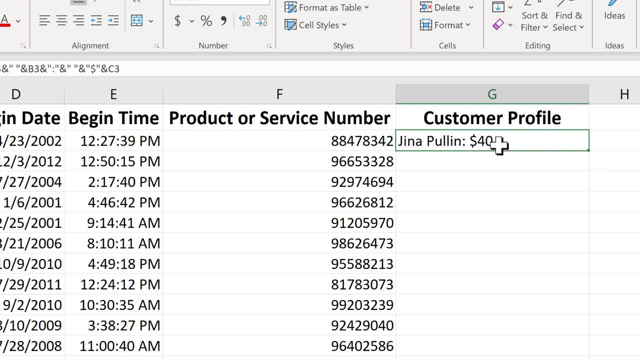 when you click and drag it, it copies whatever is in the cell that is selected. now, sometimes it doesn't just copy, it extends. and if you haven't watched my tutorial on the autofill handle, you really need to do that. but in this case i really do just want to copy whatever. 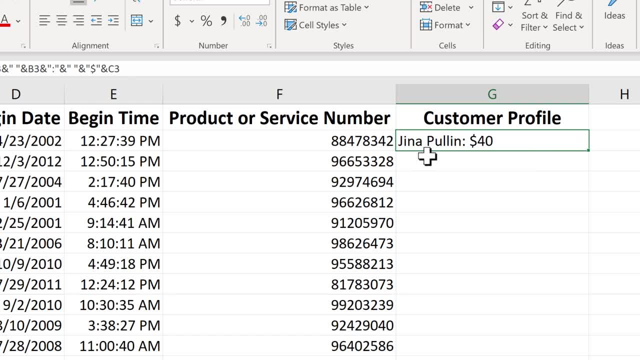 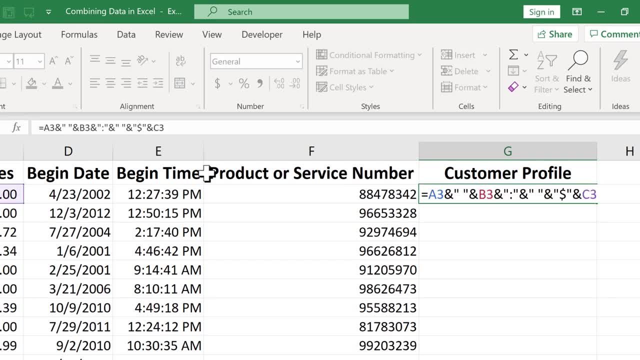 is in this cell. now some of you might say, no, you don't. you don't want to copy gina pullen forty dollars. well, if you think about it, that's not really what's in this cell. if i double click on that cell or if i just click on it once and look up here at the formula bar, you can see that. 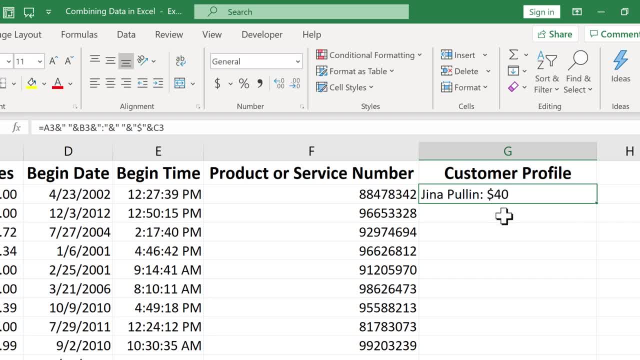 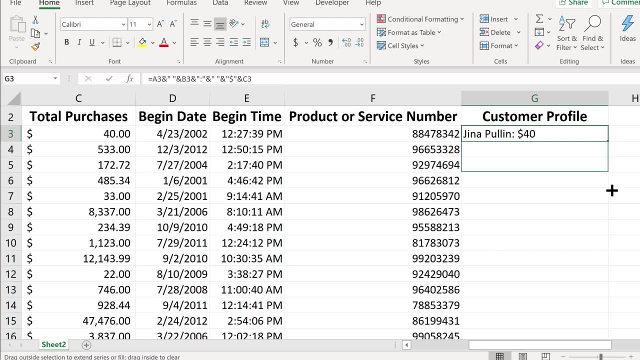 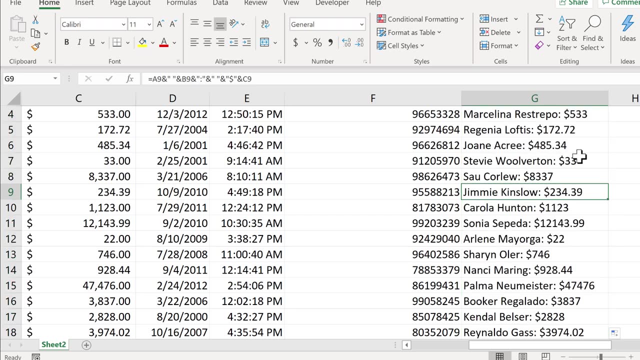 this is actually a formula. it's not just gina pullen forty dollars. so i want to copy that formula down this column. so i'll click and hold that autofill handle and just drag down the sheet and release and look what it did. it combined the first name, the last name and combine that with the. 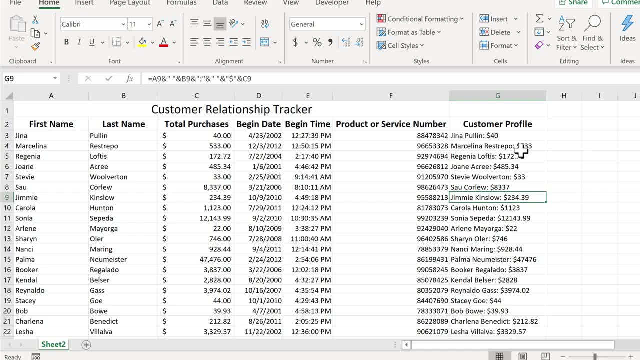 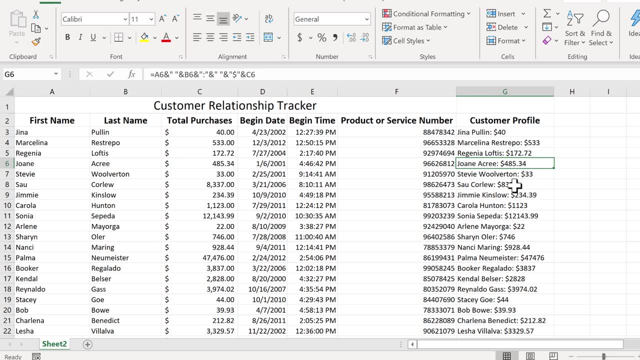 total sales, and that's what i'm going to do now. i'm going to go to the autofill handle and i'm going to drag down the sheet and i'm going to add the total sales from each customer. now just one thing to take note of the results. here in column g they end up being treated like text, so these aren't. 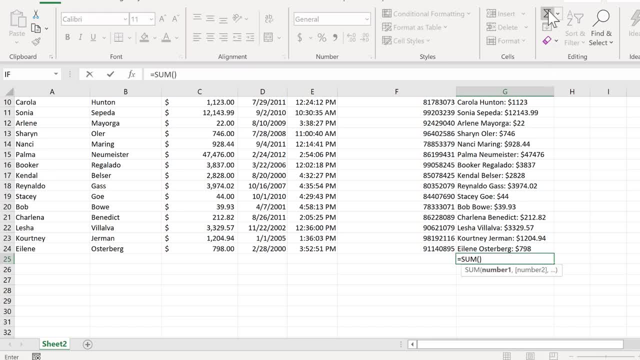 really numerical. they have numbers included, but if i were to do an auto sum, it doesn't really know how to handle that because these aren't really numbers. they're just formulas that combine text with numbers and the result is treated basically like text, and i really think the more you use 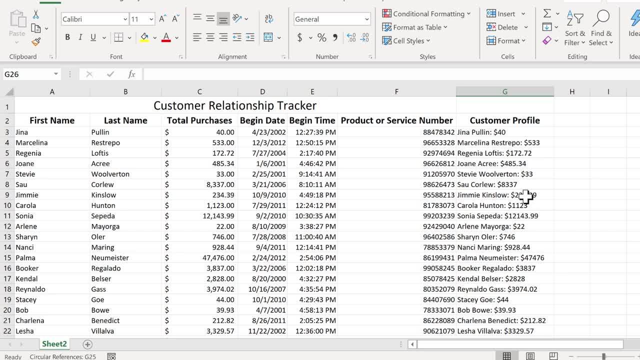 the more you'll see opportunities to use the ampersand to combine data from more than one cell and pull that data together into one cell. thanks for watching. i hope you found this tutorial to be helpful. if you did, please click the like button below and consider connecting with me on. 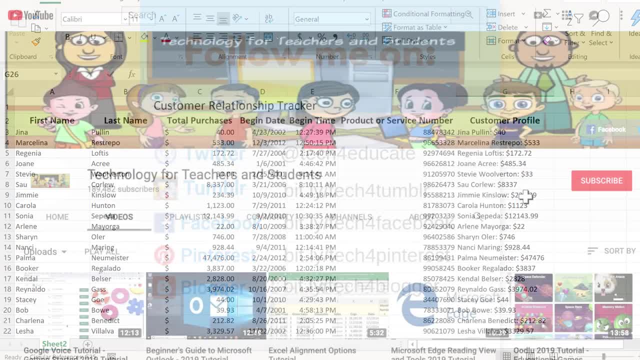 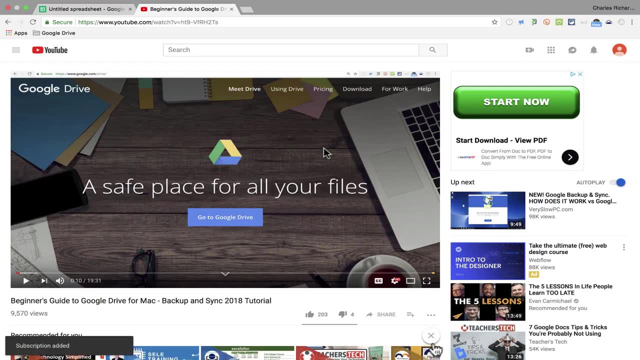 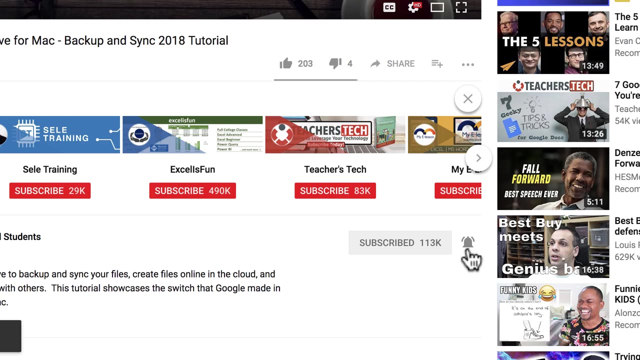 my social media accounts like facebook, pinterest and twitter, and definitely do subscribe to my youtube channel for more videos about technology for teachers and students, and when you do subscribe, consider clicking the bell next to the subscribe button. you'll be notified whenever i post another video, and watch for another video from me, at least. 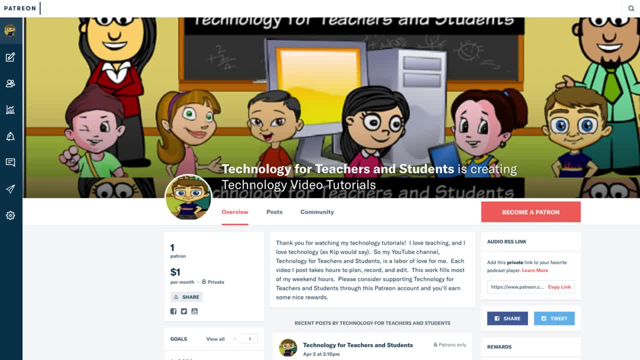 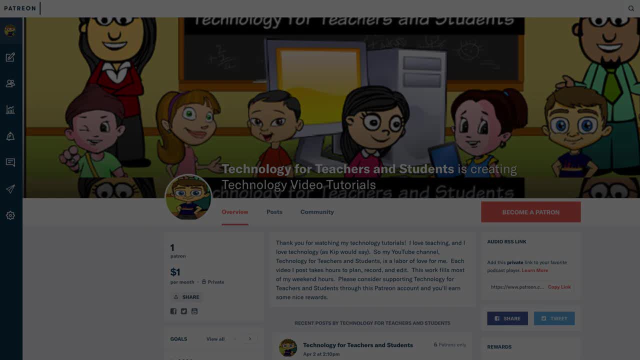 every monday. if you'd like to support my youtube channel, consider becoming a supporter of mine through my patreon account, and you'll see a link to that in the description below. 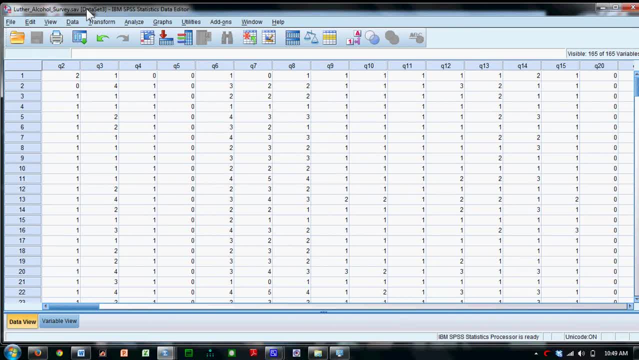 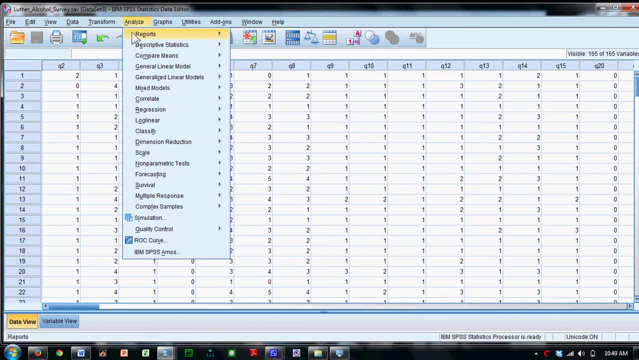 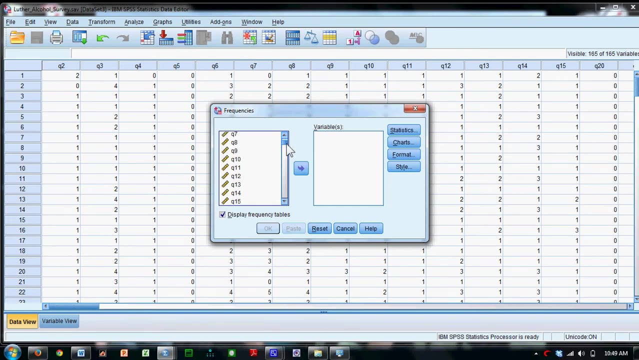 So I've got the Luther alcohol survey data open and what I want to do is come over here to analyze down to descriptive statistics, over here to frequencies. Now I'm gonna have to scroll down quite a ways, but I get down here and I find four variables: audit caps, depress and PSS4.